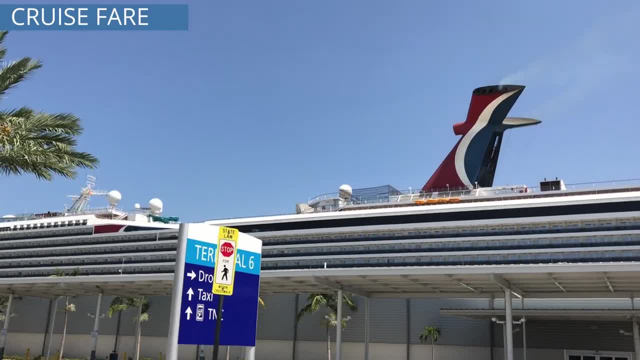 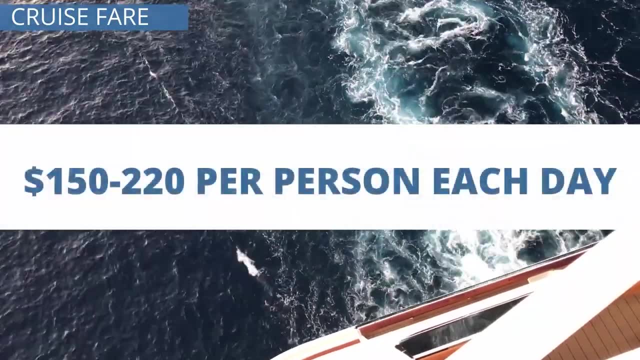 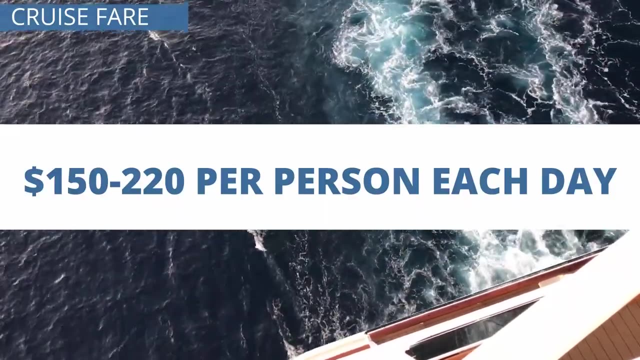 passenger statistics. That gives some insight into what people spend on average. From these public reports we note the average cost of cruise fare runs from about $150 to $220 per person per day, depending on the cruise line. For example, in 2019, the last full year of sailing Carnival Corporation. 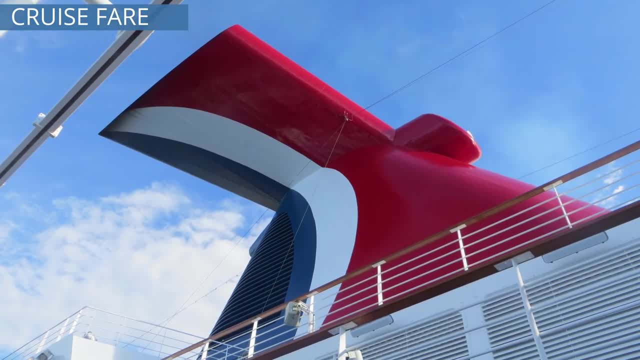 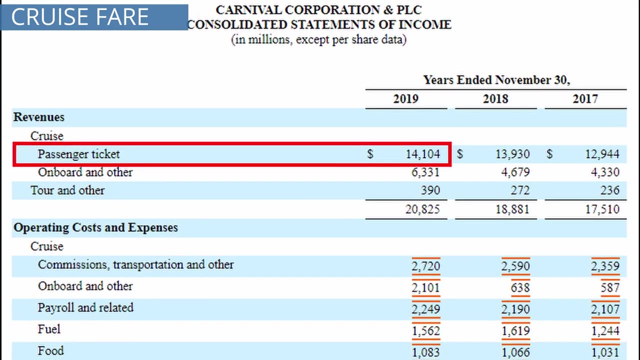 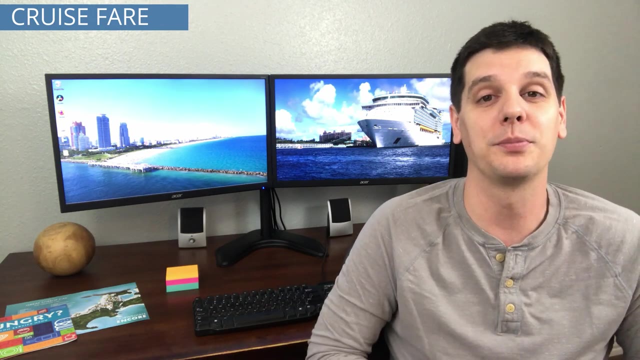 which owns several different lines, took in $14.1 billion in ticket revenue and sailed 93.4 million passenger days. That comes out to $151 per person per day. Of course, those figures can be much lower or much higher, depending on your specific cruise. For example, sailing in an interior cabin is drastically cheaper than sailing in a balcony room, and cruises departing in January or February are less expensive than those sailing at the height of summer. Still, these figures should give you a good idea of what the average cost of your cruise. 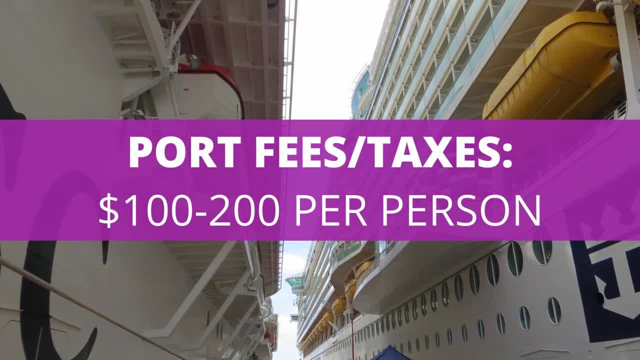 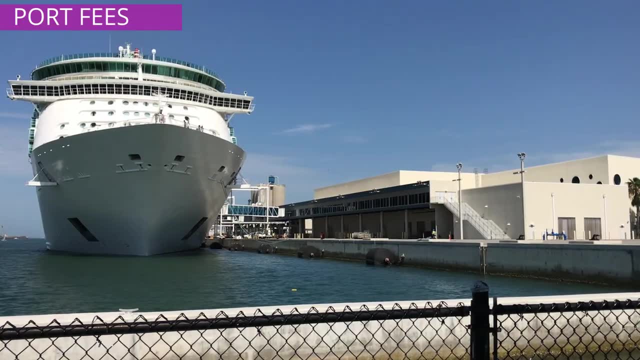 is based on what others pay. Port fees and taxes aren't technically part of your cruise fare, but they are included in what you pay before you board. These costs don't go to your cruise fare, but they are included in what you pay before you board. 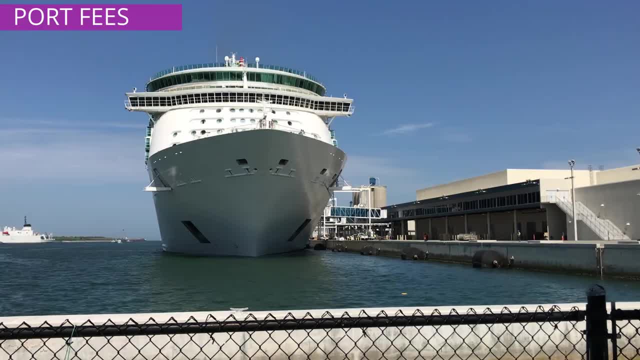 Port fees and taxes aren't technically part of your cruise fare, but they are included in what you pay before you board. These costs don't go to your cruise fare, but they are included in what you pay before you board. So how much will you pay for these port fees? The amount varies depending on your specific. route, as different ports charge different fees. In my experience, most cruises expect to spend between $100 to $200 per person on these fees and taxes for your entire trip. Some cruises with fewer ports will be less money As a rule of thumb. 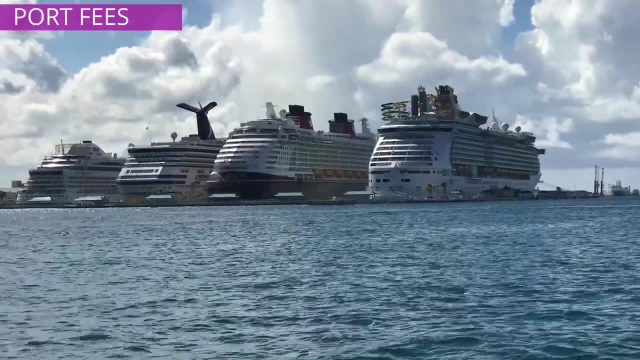 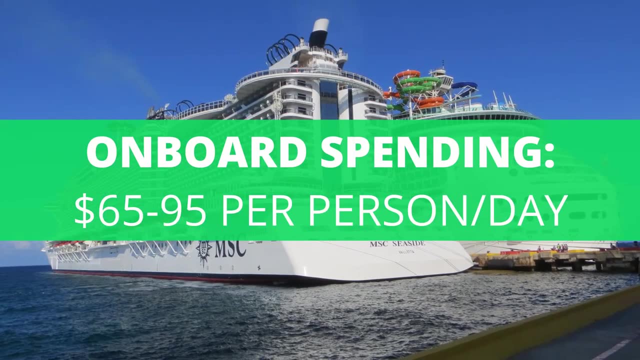 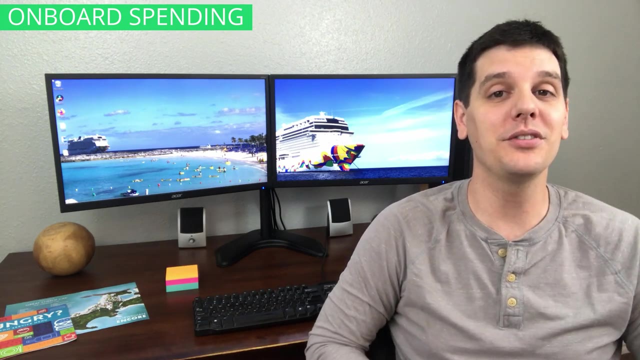 the more ports your cruise visits, the higher the port fees you should expect. If you want to save here, then look for shorter trips with fewer stops. By far the biggest expense of taking a cruise is the cruise fare, but onboard spending comes in. 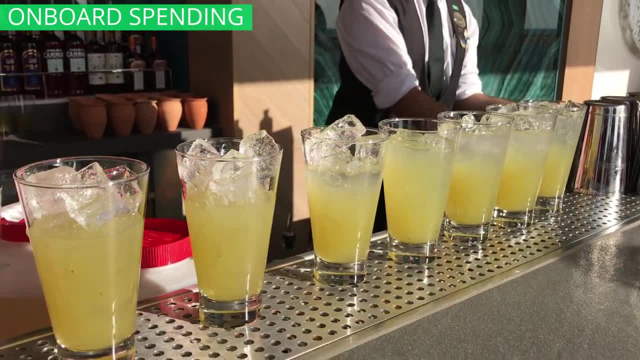 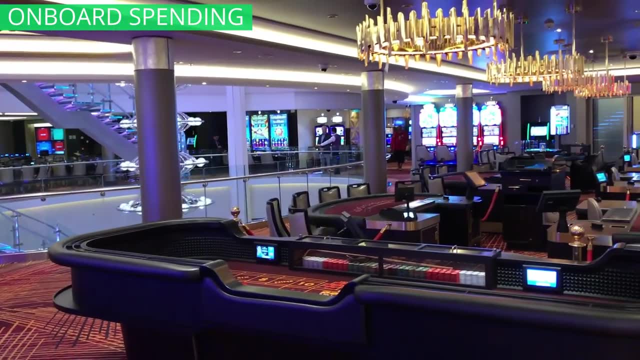 second for most people. So how much will you spend once you're actually on the ship? Along with cruise fare, the cruise companies break down how much cruise passengers spend aboard the vessels within their financial reports. On average, across cruise companies, the amount comes out to: 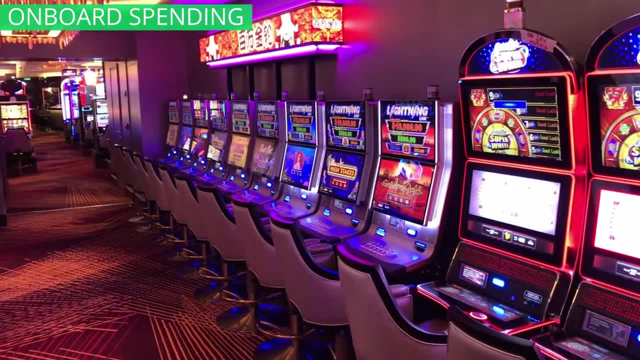 around $65,000 to $90,000 per person per trip. That's a lot of money for a cruise, But if you're an onboard hospice, then checking the horoscope will never come to much of a difference. Carnival Corporation reports the lowest amount of onboard onboarding spending. 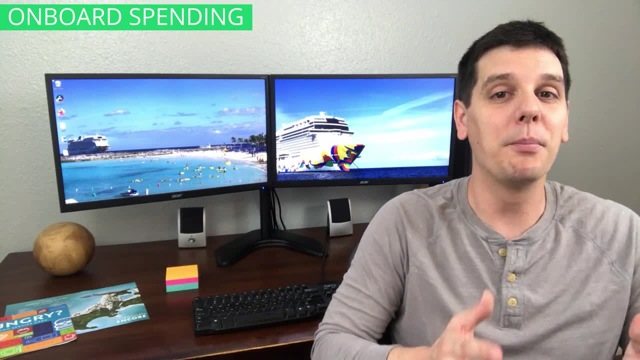 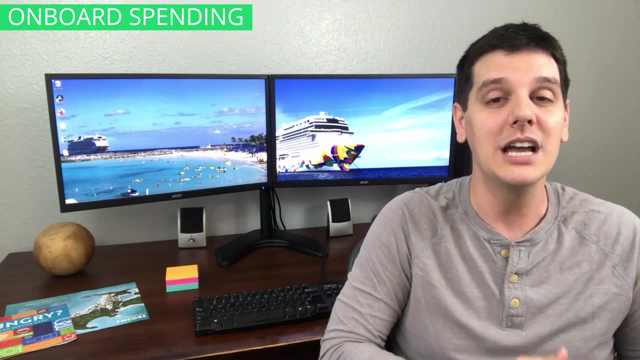 while Norwegian Cruise Line Holdings the parent of NCL reports the higher amount, It's common to spend 30-40% of what is spent on cruise fare just on onboard spending. Keep in mind that this is simply an average across all cruise. 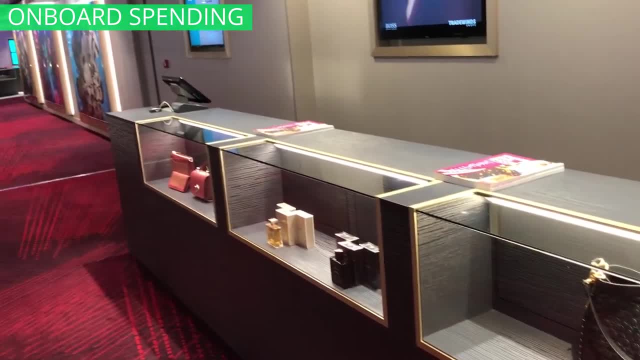 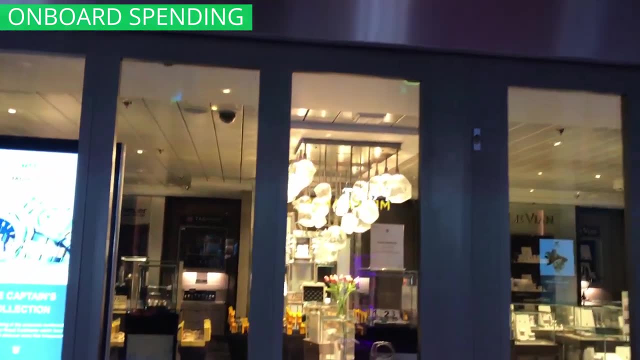 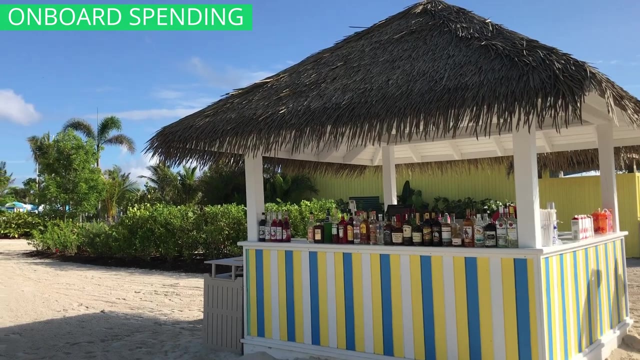 passengers and major cruise lines, What you spend could be drastically different. Onboard spending is the one area of your trip where you are in complete control of how much or how little you spend. For instance, some people spend little or no money once they're on the ship. 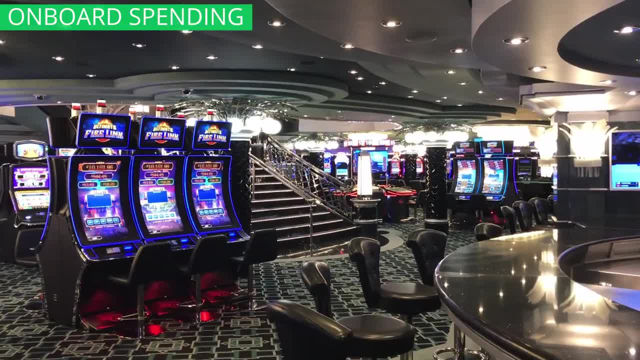 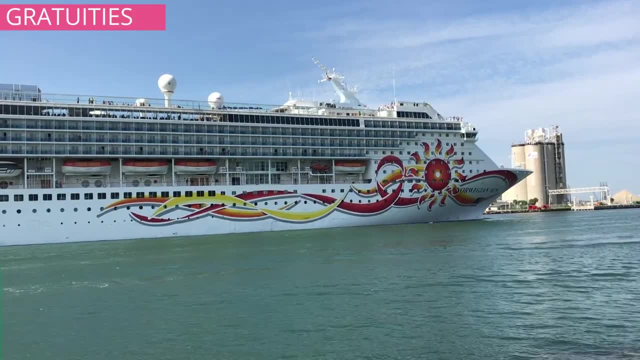 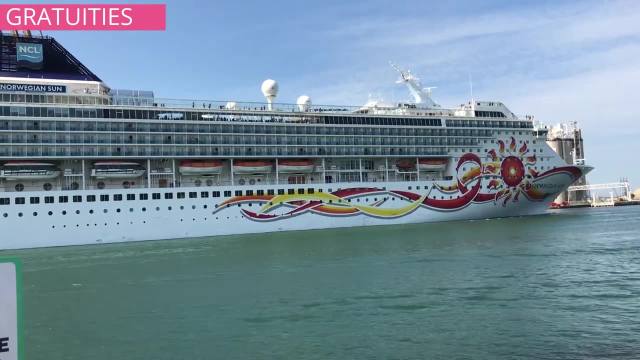 Others purchase things like drink packages or they gamble on the casino and generally live it up for the entire cruise. Gratuities are a fact of life on a cruise ship. Yes, you can adjust the amount of gratuities if your service is particularly poor, but 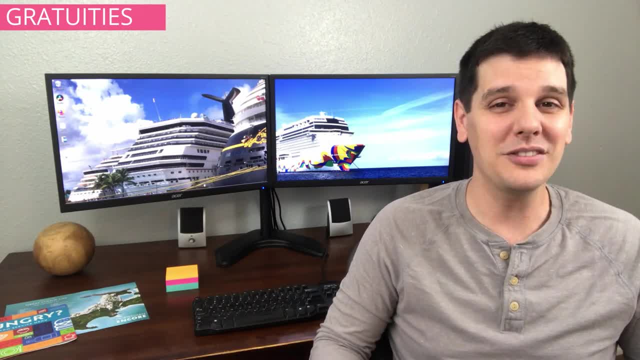 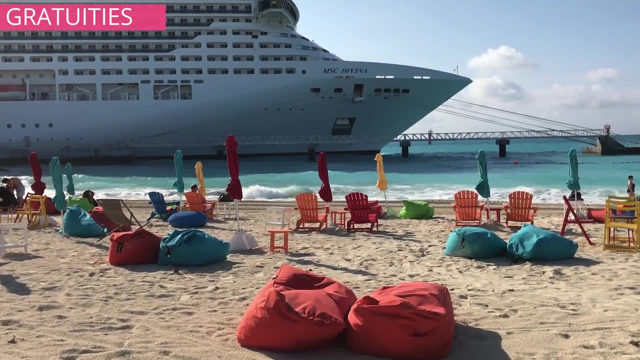 for most of us that's not something that's going to happen. Expect to spend about $15 per person per day, so a couple traveling on a 7-day cruise will spend more than $200 on these tips. Gratuities may be slightly higher or lower depending on the cruise line. 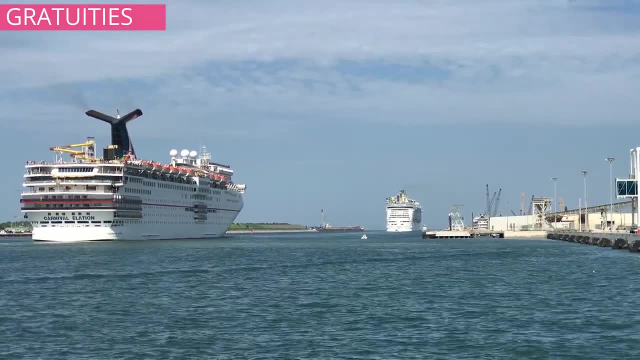 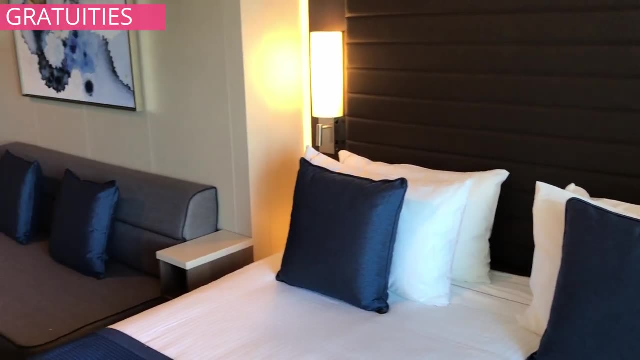 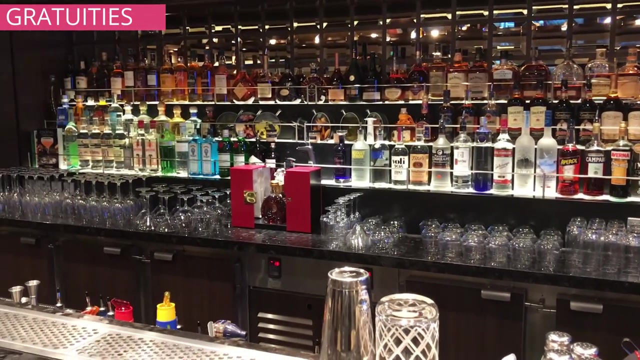 As well. guests sailing in suites have higher gratuity rates compared to lower-tier cabins like the interior or the balcony. One thing to keep in mind: this amount doesn't include the gratuities charged for extras like alcoholic beverages on the ship. Those are extra in addition to the automatic gratuities. 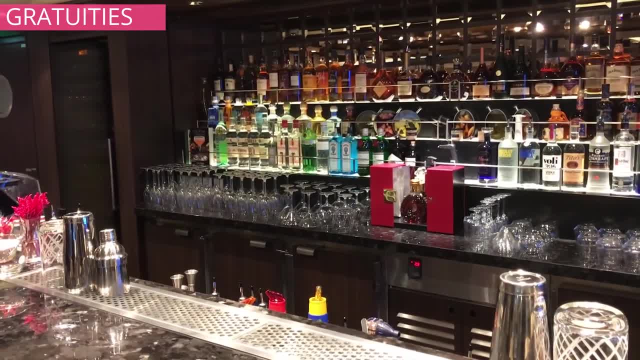 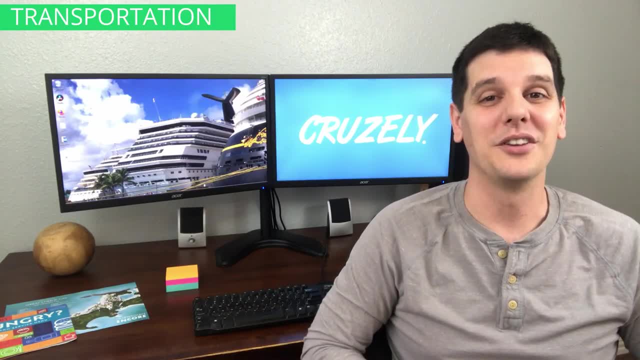 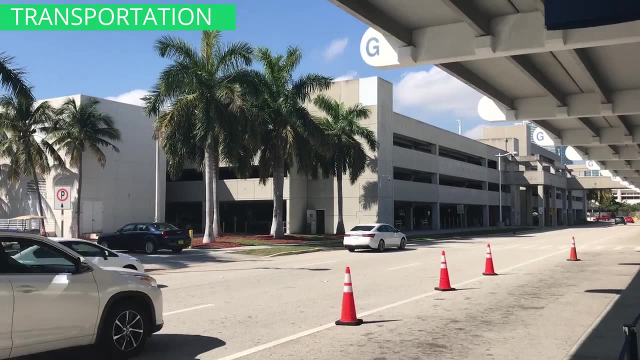 charged to each passenger that go to the waitstaff and the room steward. It's not just your cruise that costs money. There's also what you'll spend before you even get to the port, The amount that it will cost you to get to the ship park or hotel. 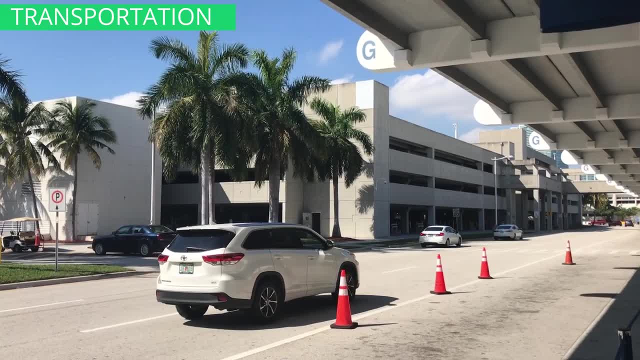 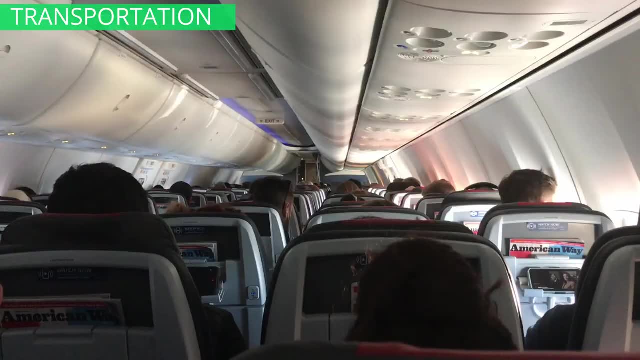 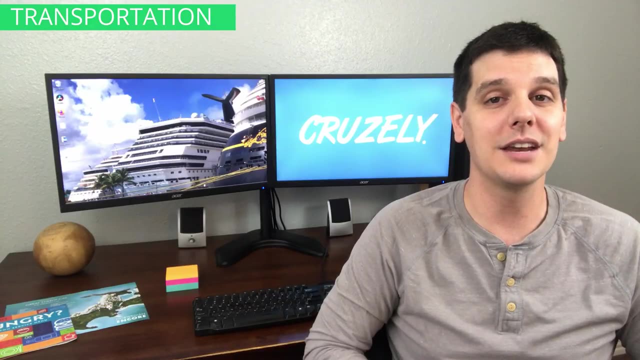 stay will vary based on your needs. Some people live near the port and just get dropped off at the port by a friend or an Uber. Others have to book cross-country flights and a hotel stay the night before. If you drive to the port, plan to spend around $20 per day for parking, depending on the actual 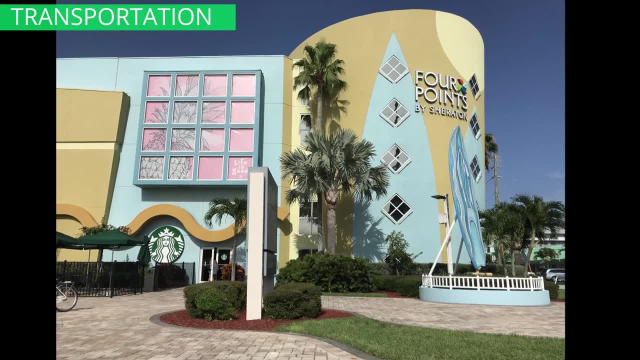 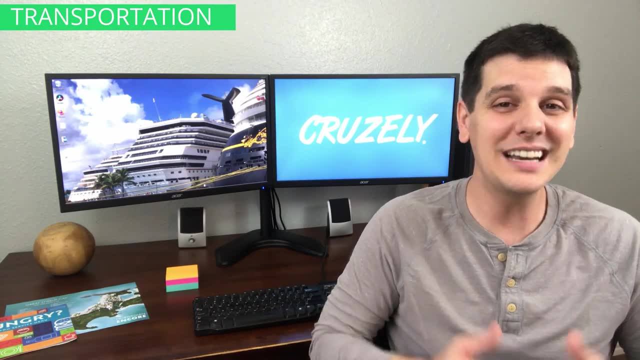 cruise port Hotels in most cities can be found between $100 and $200 per night. Rides to the port or the cruise terminal using services like Uber or Lyft can vary considerably depending on where you're coming from. Still, you don't want to forget these considerable. 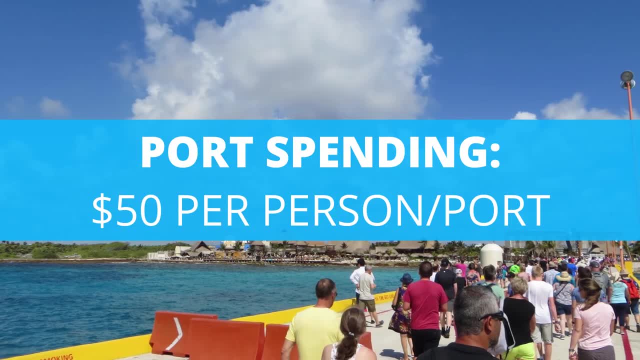 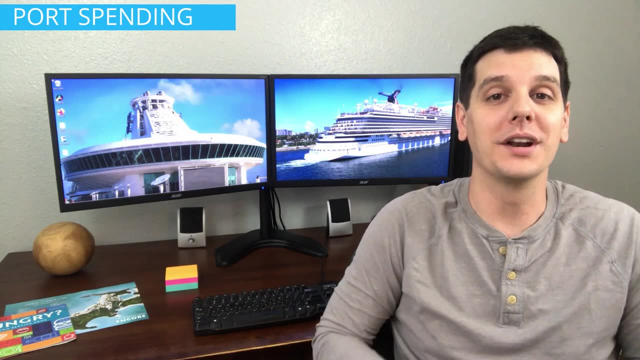 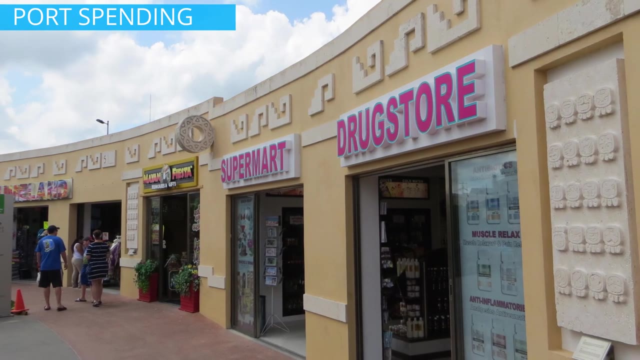 expenses and budgeting for your cruise. Finally, let's talk about spending in ports of call. What you spend in port can vary widely. Remember: anything you eat or drink off the ship will come out of pocket and isn't included in your cruise fare As well. things like taxis and souvenirs are also extra costs. As a rule of thumb, I like to estimate a budget of about $50 per person per port of call. For some ports that may be too much. For instance, at Cruise Line Island, they often have what you need already included. Other ports might include a stop at a restaurant, some souvenir shopping and buying drinks. 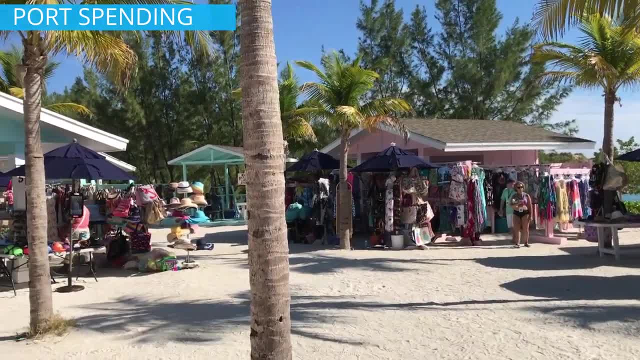 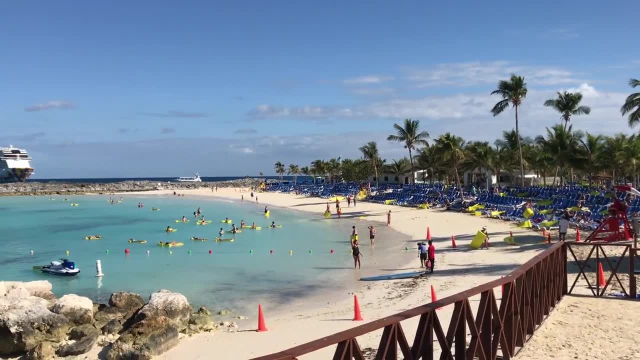 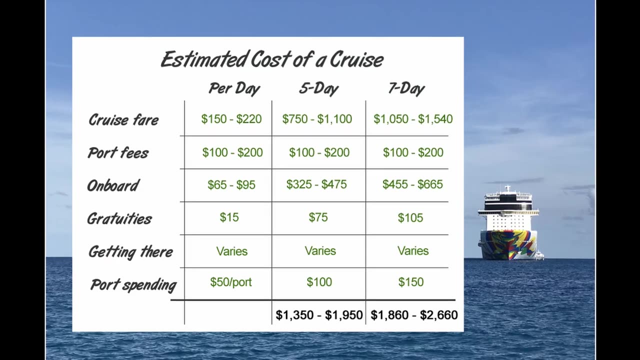 at a bar on shore. These costs can quickly add up. So what's the grand total? Adding up all of these expenses that I've covered comes to a per-person estimate for what you can benchmark for your cruise. As you can see, for a 7-day cruise, it's about $50 per person per port. As you can see for a 7-day cruise. 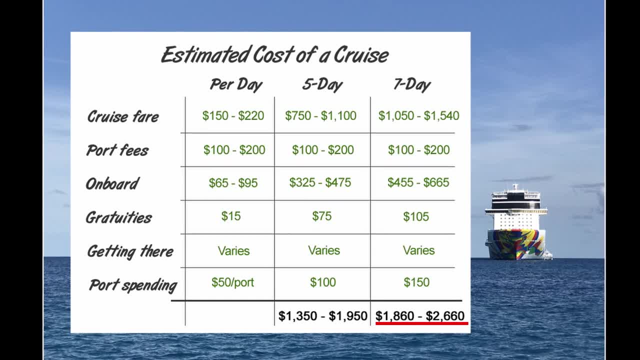 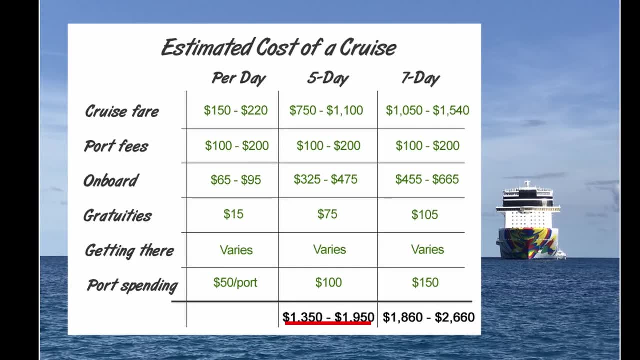 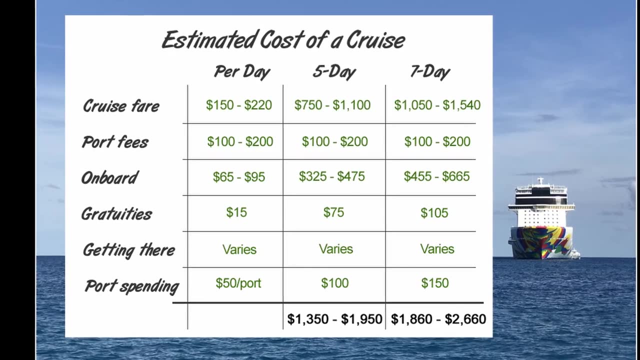 you can expect to spend around $2,000. when you factor in everything For a 5-day cruise, that figure is closer to about $1,500.. A couple would expect to double these prices. If those numbers seem scary, do not worry, These are just estimates and you do have. 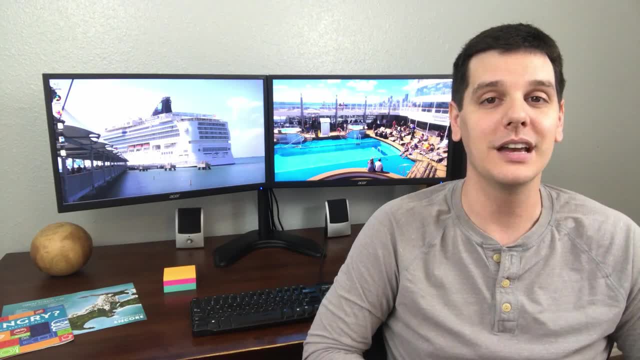 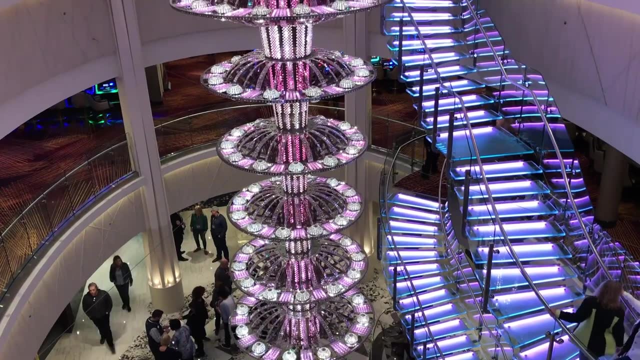 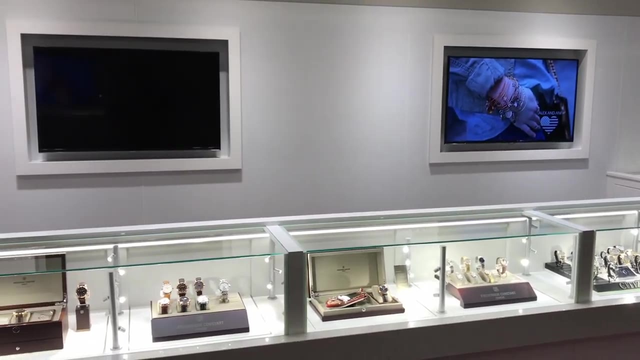 a lot of individual control over what you'll spend. For instance, sailing off-season in a lower-tier cabin or on an older ship can drastically cut your cruise fare In onboard spending. as I mentioned, it's the largest expense outside of cruise fare. 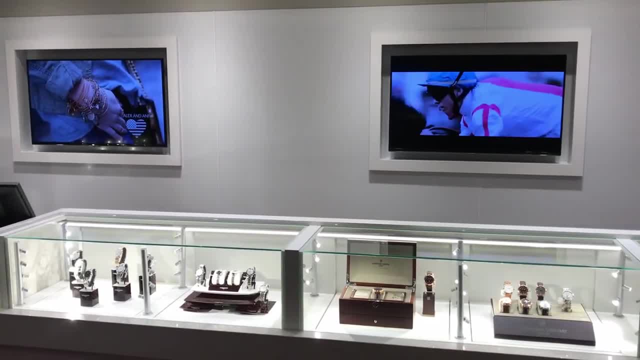 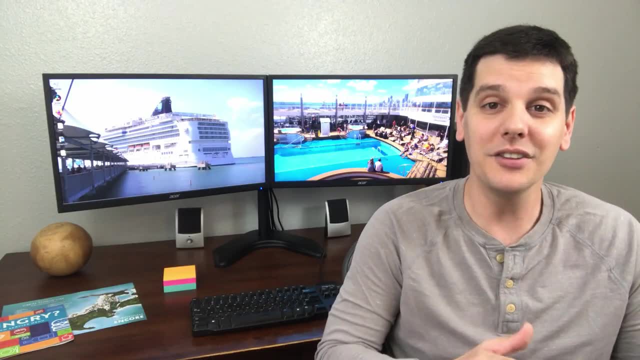 but it is optional. You can sail without spending another dime if you want to. In other words, if you want it to be, cruising can be amazingly affordable. On the other hand, if you want to splurge on things like suite cabins and high-end restaurants, then you can spend as 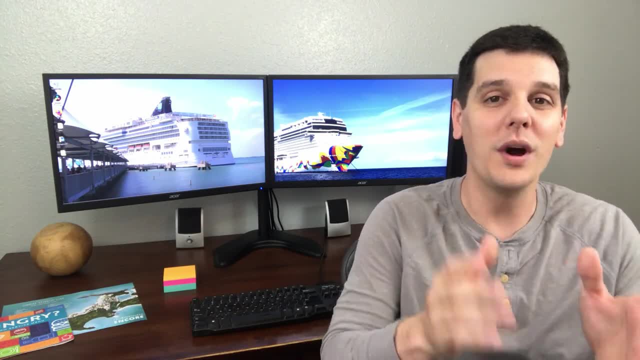 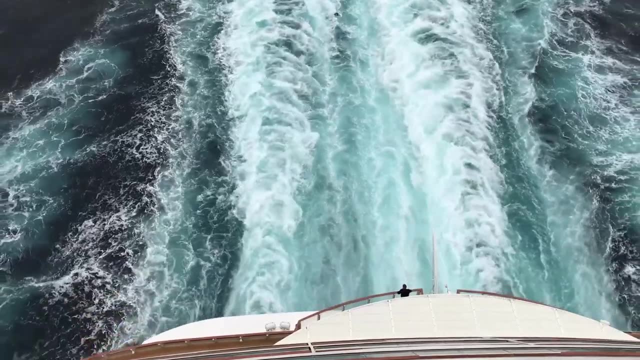 much as you want. The good news is, what you budget is in your control. Thanks for watching. I hope you have a better idea of what a cruise might cost you Now. if you liked this video, be sure to like it, and you can also subscribe As well. check. 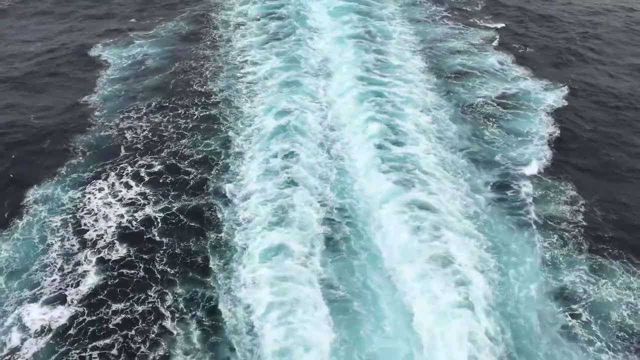 out our channel for more helpful videos on planning your cruise. Until next time, happy cruising.